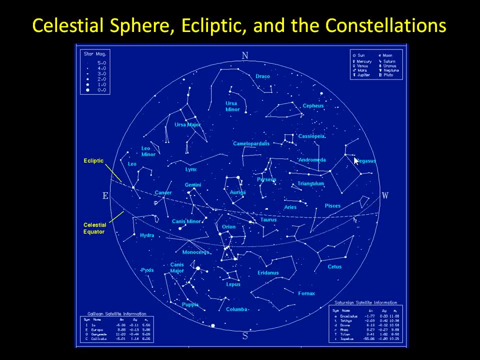 these patterns, which we call constellations. It's very useful and it's been used for many years. In the past, people have assigned special stories to these constellations. When you look at these groupings of stars in the night sky, it's very important to keep in mind that there's not 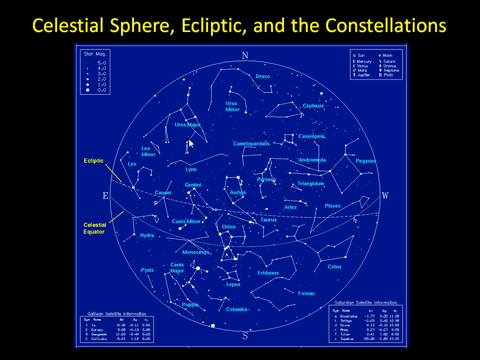 really any significance to their relative location to each other, because you're looking at a projection. When you look at any given constellation, the stars that make up that constellation are all at completely different distances, Even though they look like they're right next to each other. as viewed from earth, they could be at very, very different distances. 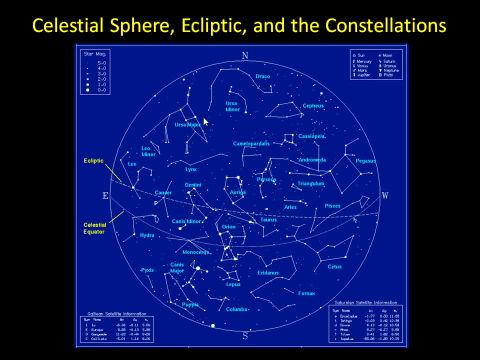 from earth and they really have no relation to each other. It's just how they appear from our location. Another thing to keep in mind: when you look at the bright stars in the night sky, you're typically looking at stars that are a few hundred to a handful of thousands of light years. 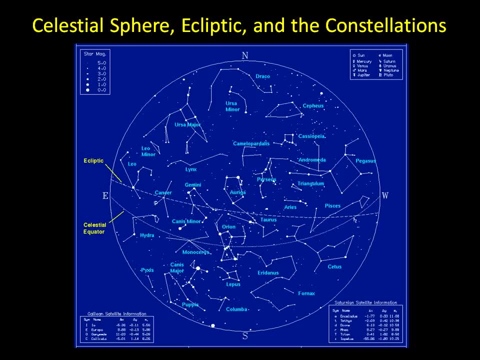 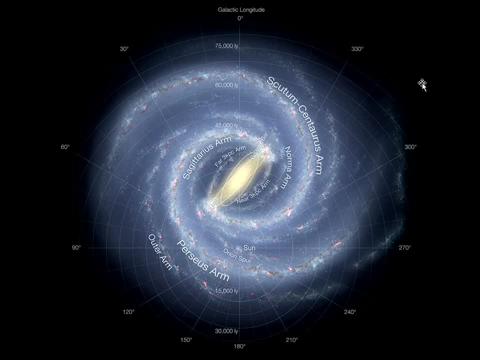 away To put that into perspective. look at this. This is a cartoon of the galaxy that we live in. I know we haven't really discussed this. Let's talk about the stars to the last minute. I know that some of these stations aren't quite as good applicants now as the stars we mention today. 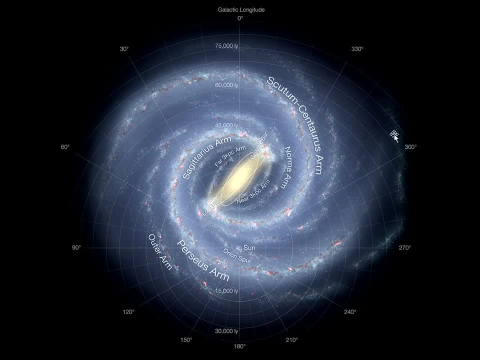 are, though, for keeping in mind the stockings on earth. The galaxy is crammed in hundreds of billions of stars, like the sun and arms. including the sun. we orbit, and we can see these interacts in calm layers of light, where the stars are many times focused. 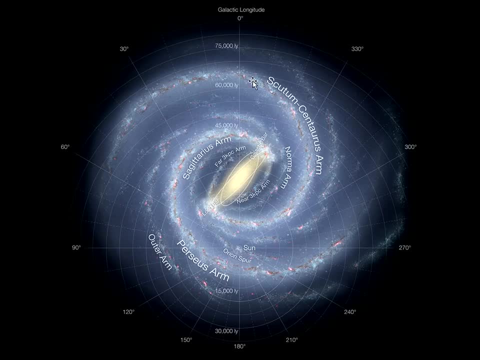 The stars are also compressed into and flattened in pancake shape. So when you all saw the creation of our galaxy at night sky, it couldn't have been more interesting to see, because you don't know how much light was taken from a galaxy at. 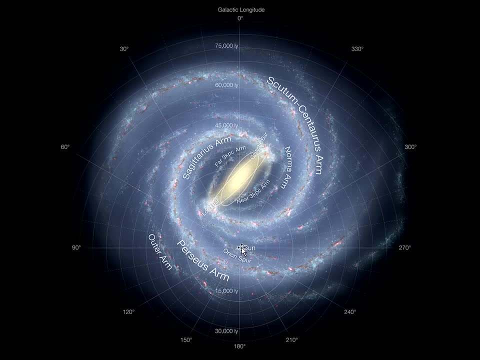 all immediately, And another thing that really resonated with me about this was that there are thousands of stars as caught in these arcades And it can be deadly, And that especially has to do with theius clock scientists And that's just looking at this little neighborhood of the galaxy that we're in right now. 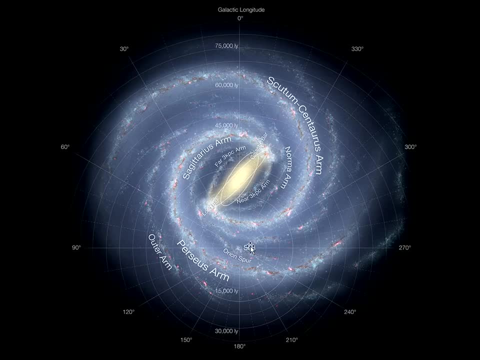 The galaxy itself is about 100,000 light years in diameter. So when you're looking at the stars in the night sky, you're just looking at the stars in our neighborhood right here. You can't see these stars that are much further away. 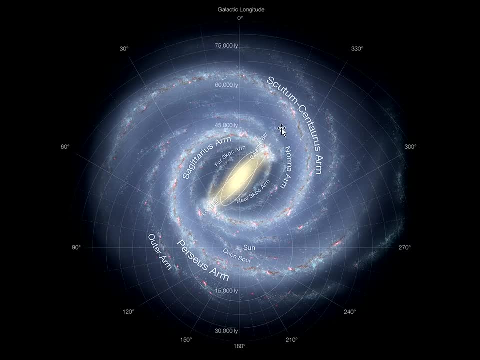 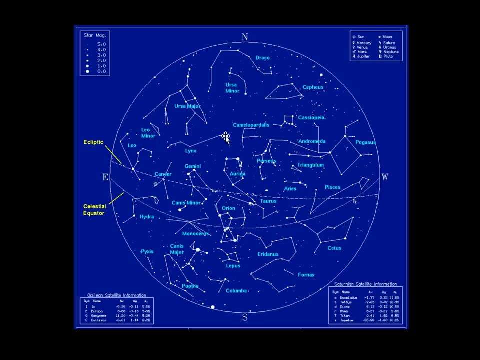 There's gas and dust, which obscures our view, So keep that in mind when you look at the night sky. You're just looking at relatively nearby stars relative to the size of our entire galaxy. There's a couple other features that I want to point out in this star map here. 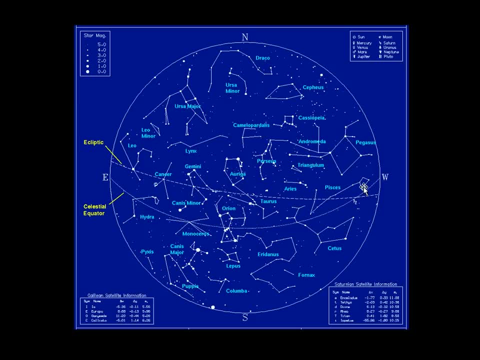 There's this thing called the ecliptic and there's this thing called the celestial equator, And both of these are located fairly high in the sky. So this is your northern horizon, Your western, southern and eastern horizon. This right here is looking straight up. 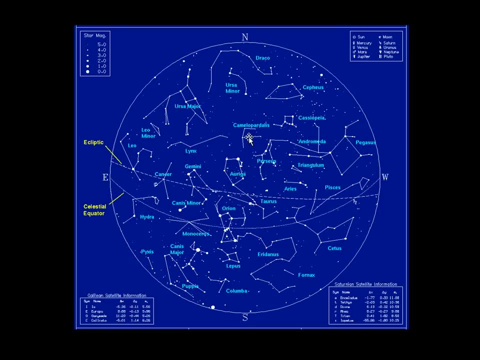 And you see, the ecliptic and the celestial equator are pretty high up in the sky in the star map, And this is what we want to really understand in this video today: These constellations that you see on any given night. this is just a fraction of the total number of stars that are visible from Earth. 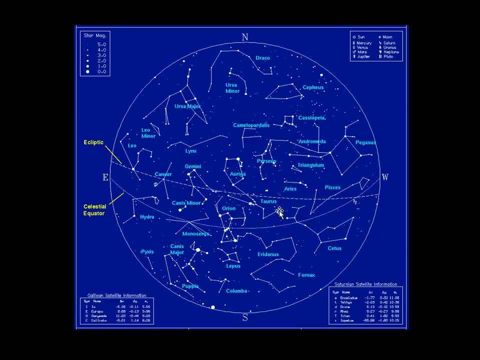 Some stars are only visible at night. Some stars are only visible at night during the winter, And other stars are only visible at night during the summer. And also there are some stars that we never see from a place like Ventura, because they are only visible from the southern hemisphere. 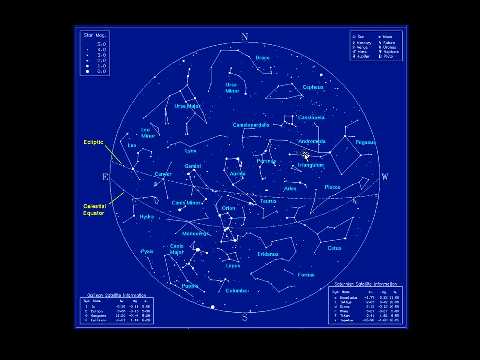 So you'd have to travel south of the equator to see other parts of the night sky. But if you piece all of that together- all of the night sky visible different times of the year and visible from the northern and southern hemisphere- you'd have to travel south of the equator to see other parts of the night sky. So you'd have to travel south of the equator to see other parts of the night sky. You can break up the entire night sky among theuma of all absersers on Earth. You can break up the entire night sky among theuma of all absersers on Earth. 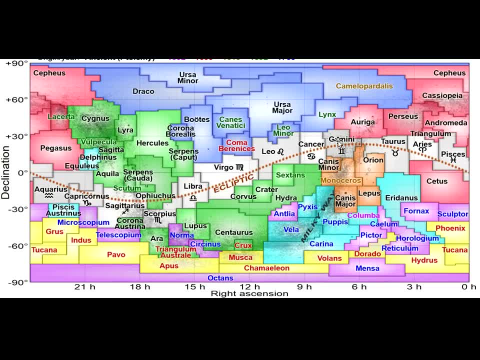 into this patchwork state of the total number of 88 constellations. So astronomers have agreed to take the entire sky and break it up into 88 patches And they all have names And deal. they are Alright. so there are the 88 constellations. 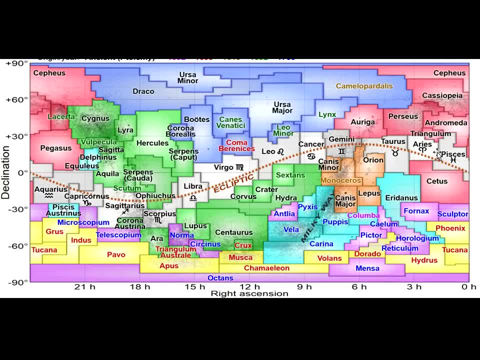 A little sneak preview over here. This thing called the ecliptic, which I'm about to explain, This thing called the ecliptic, which I'm about to explain. you notice that the constellations that line up with the ecliptic, these are probably the ones. 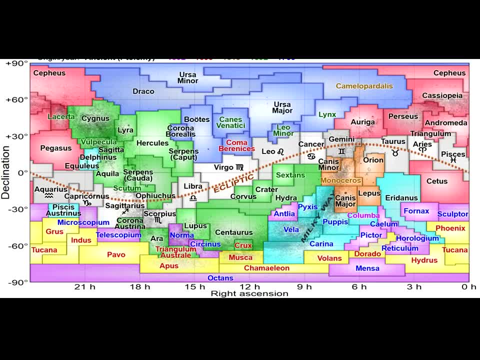 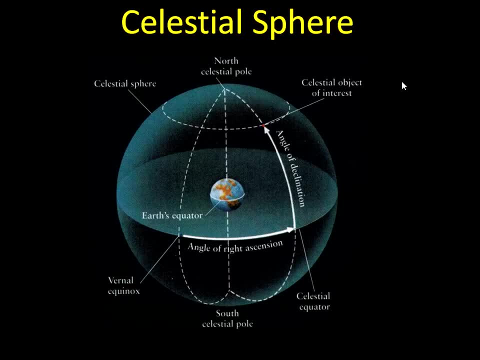 you've heard of, these are the constellations of the zodiac and we'll say a few words about that in a second. so this concept of the celestial sphere which we introduce in chapter two, this is very important in in both this chapter and the upcoming chapter, chapter three, when we include the 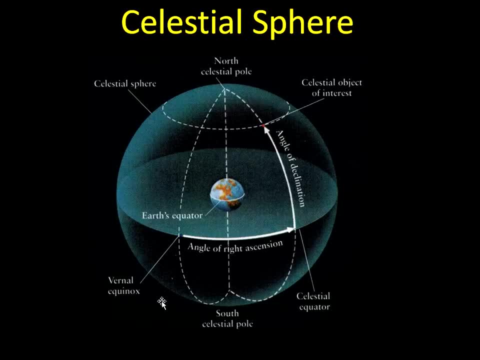 moon, and this is this not something that's real, but it's, it's a useful tool in astronomy. we are, of course, located here on earth, so this is where we observe the stars from, and what we do is we imagine that the stars, since they're all at these enormous distances- 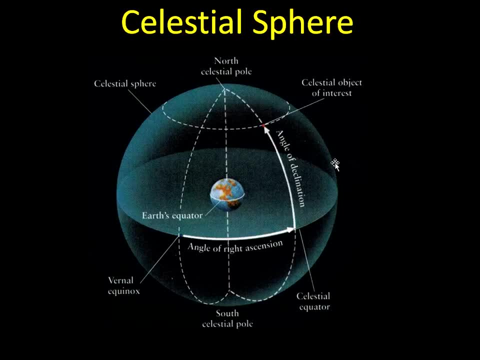 just in terms of the way that they look from earth. we can imagine, even though, again, this is not real, that the stars are all located on this imaginary sphere, and the stars are so far away that so that their relative pattern next to each other it basically remains fixed, which is the pattern. 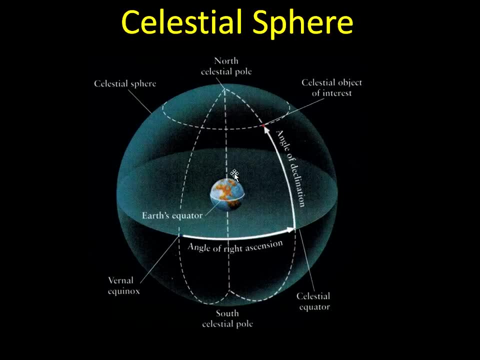 of the constellations and then, as the earth rotates, at the center, it appears as though these more or less stationary stars, it appears as though they are the things that are orbiting, even though it's really us. we are the ones that are rotating on the earth due to the earth's rotation, and so 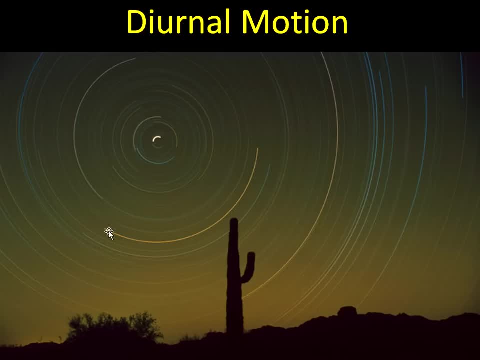 this is what the stars look like throughout the night- be due to the earth's rotation. there's something called diurnal motion. so if you were to look in the northern sky, you would actually, and if you were to keep track of the stars throughout the night, you actually see that they trace out. 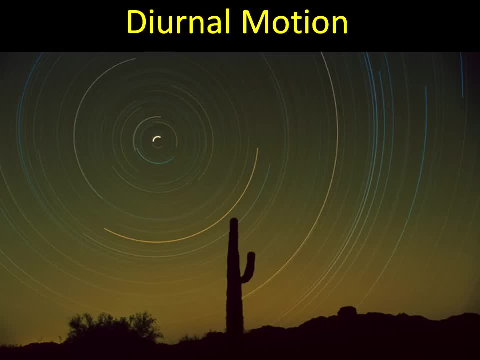 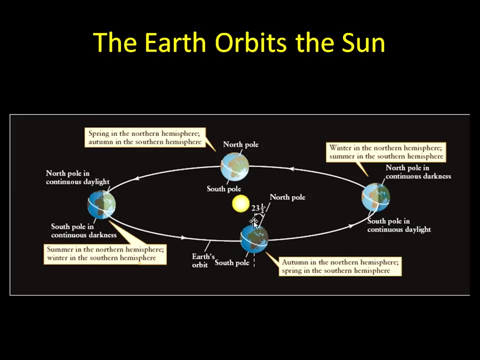 these paths. this is a long exposure photograph right there. all right, let's get to the, the ecliptic. so here is a cartoon out of our book and this shows the sun and it shows the earth orbiting the sun and if you imagine that the distant stars are out here. so 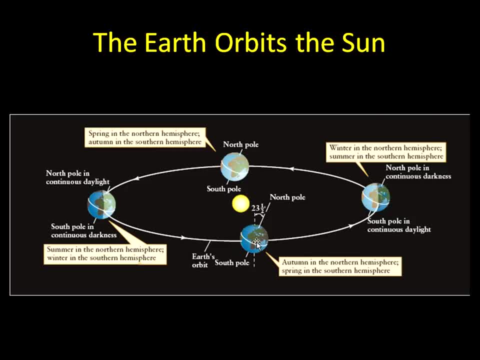 the celestial sphere is even further out as we orbit around the sun. different times of the year, the sun from uh, from our vantage point, the sun lines up with different parts of the ecliptic. and as the earth moves around the sun, as it orbits the sun, the apparent location of the sun as it 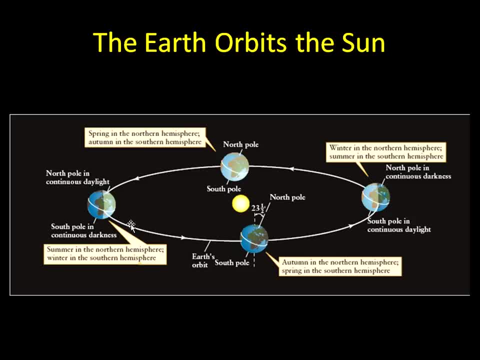 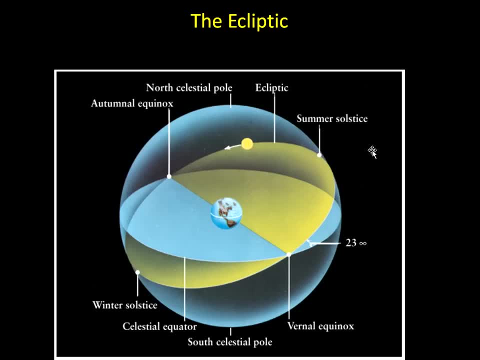 lines up with the celestial sphere. the sun appears to move around in a circle throughout the year and that path that the sun takes is called the ecliptic. here's a nice cartoon out of the book and this shows the celestial sphere. it shows the path that the sun appears to take over the course. 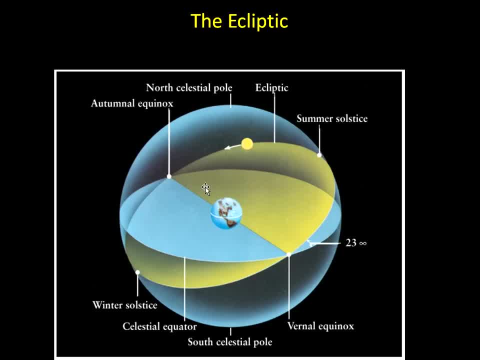 of the year, this ecliptic. right here there's another um important feature of the celestial sphere, which is the- uh, celestial equator, which is just, if you take the earth's equator and you extend it out to the imaginary celestial sphere, you have a path called the celestial equator. 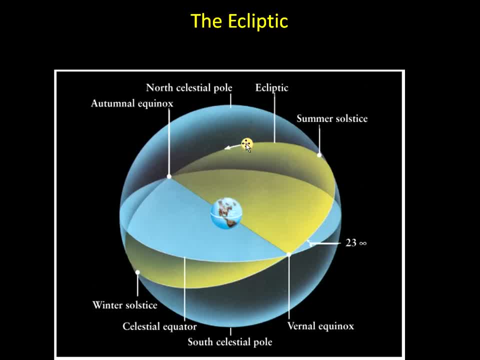 and again, the ecliptic is the path that the sun appears to take. of course that's due to the earth's motion around the sun, but to us, if we think of ourselves as stationary, it looks like the sun is orbiting us. there's two locations where the sun crosses the celestial equator: where- sorry- 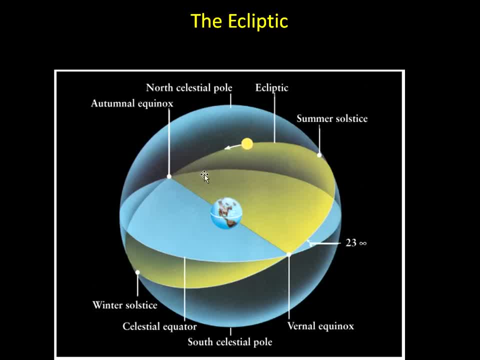 the ecliptic crosses the celestial equator. these are the two equinoxes. this is where the sun is located um on the first day of spring and the first day of autumn, and then there's these two other locations where the sun is located on the longest day of the year. 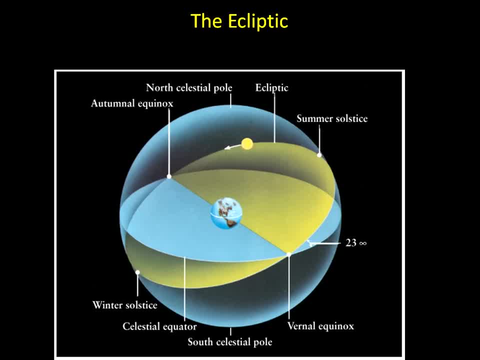 the summer solstice and the shortest day of the year, the winter solstice. so this is a very quick treatment of the ecliptic. it's a very abstract concept. you have to think about it and, you know, try to piece this together. it helps to. you know, just um, imagine what the 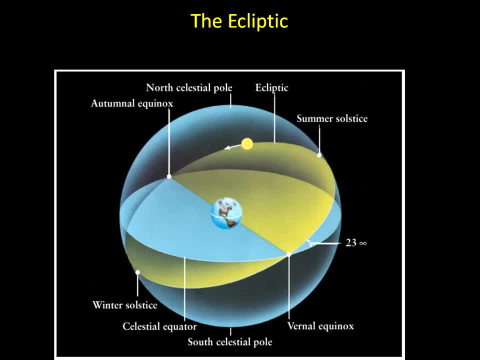 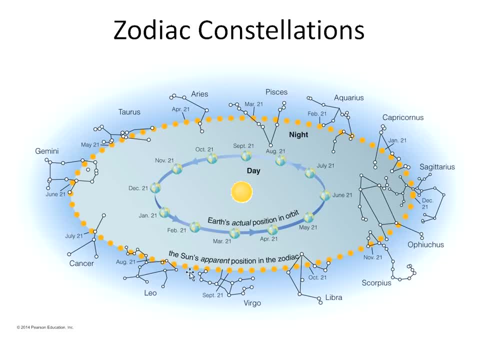 sun looks like as the earth is orbiting around it. anyways, once you have the idea of the ecliptic, then you can think about the constellations which line up with the ecliptic. these are the famous 12 zodiac constellations and in this picture right here you can kind of imagine that as the earth. 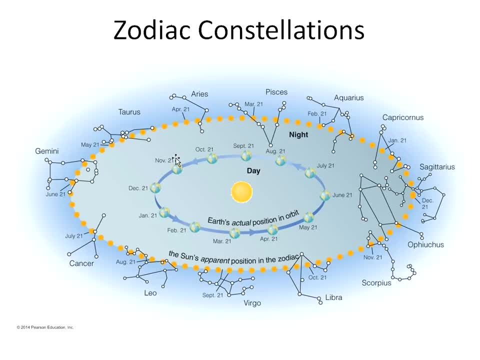 orbits around the sun. like this, different days of the year, the sun is going to line up with different constellations and this set of 12 constellations- these, these are the constellations that the sun appears to line up with as the earth orbits it throughout the year. i'm going to post another. 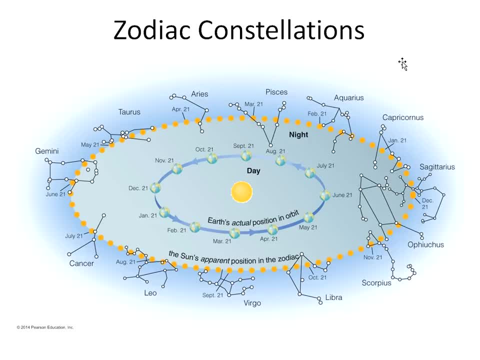 video on a zodiac constellation project and i will see you over there.